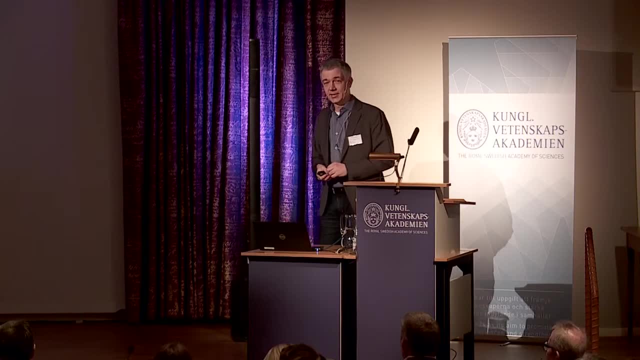 you want to be in terms of petamols, 227, is in the ocean of oxygen. The atmosphere is most of the oxygen, So 99.4%. So whatever happens in the ocean about oxygen, we will still be able to breathe for most. of the oxygen. That's the question. No negative results. Okay, So let's just add some facts. We have some more questions, because we just had the question and I was just trying to ask if you had any questions about oxygen. 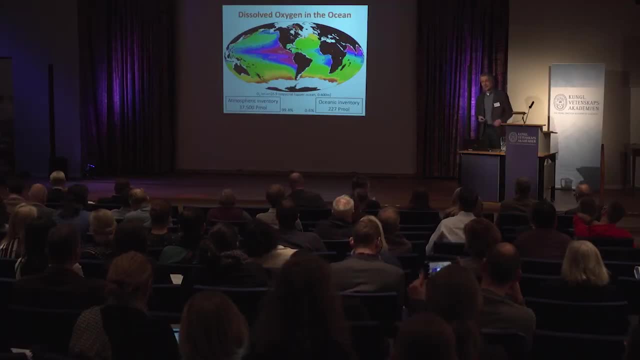 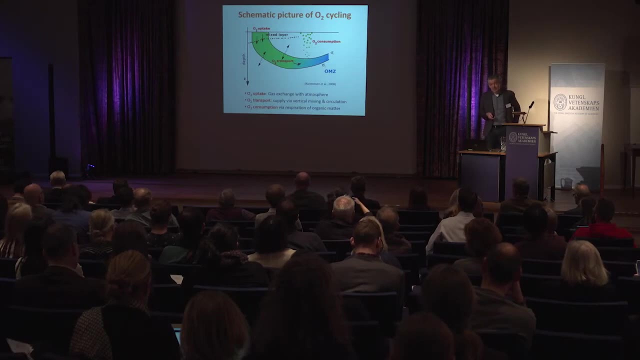 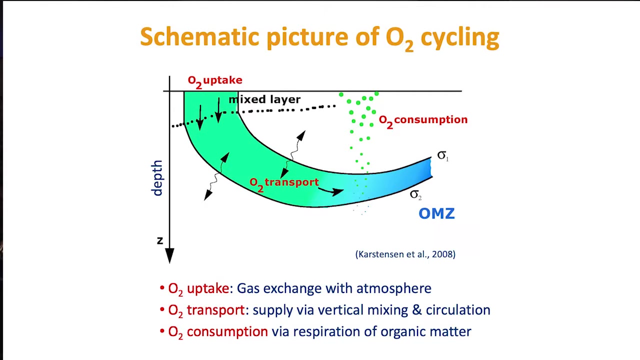 a while, a very long while. So that's, we don't have to worry from that perspective. That's the first positive news. The mechanism: how does this large pool of oxygen in the atmosphere affect the ocean? That's the interesting part here. And there's oxygen uptake at the 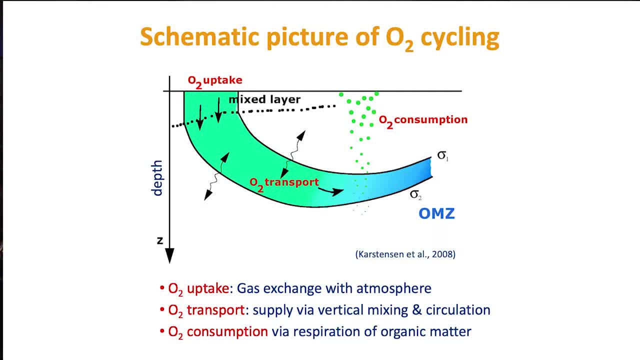 surface in the mixed layer, then transport with the ocean currents, with mixing and advection into the interior and all the way consumption, rain down of or circulation dissolved organic matter, particulate organic matter has respired and consumes oxygen away And with climate. change, and particularly global warming, we see that uptake will be reduced. That's what we expect. So less solubility. the gas, the amount of gas warmer water can hold, decreases with time. That's the champagne bottle effect. So less oxygen going in and on net, more oxygen bubbling. 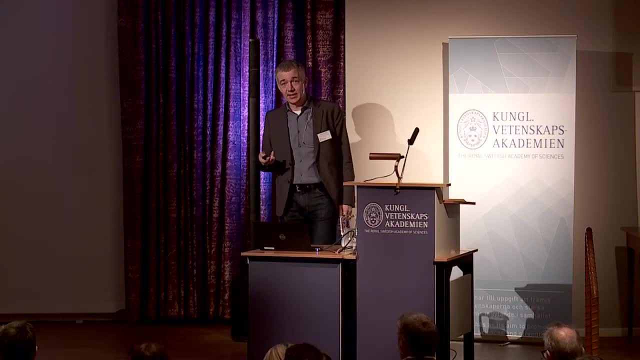 out. Second part is transport, That's. we expect that will be reduced because the ocean warms from the top, So a lid of light warm water is sealing off the ocean interior, So this transport pathway will become more difficult. We need more energy to bring water down And 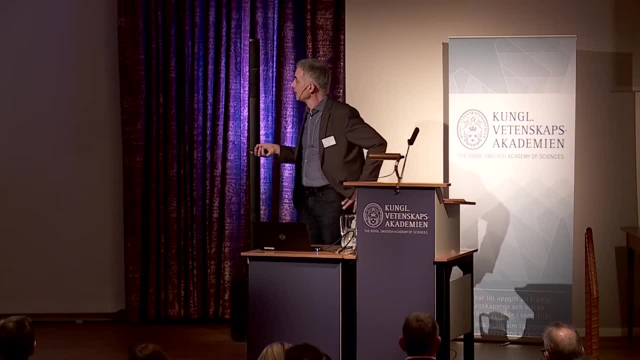 that depends on winds and so on. We will have that discussion. And then third part, oxygen consumption. That we don't know so much. So of course respiration rates will increase. That's a metabolic effect. But usually oxygen consumption in the global ocean is not rate limited, It's substrate limited. So it depends on how much organic matter we form And this depends on how much nutrients can be brought into the light, And that might well go down because there's less production and less nutrients coming through. 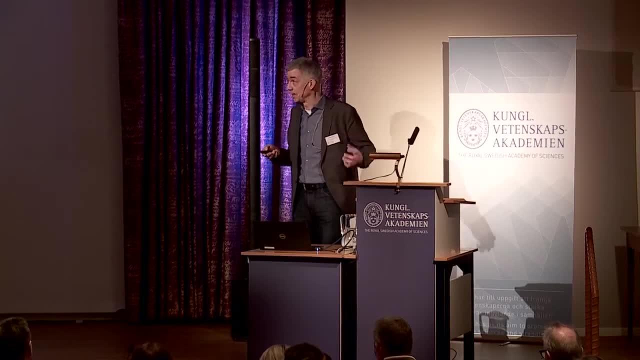 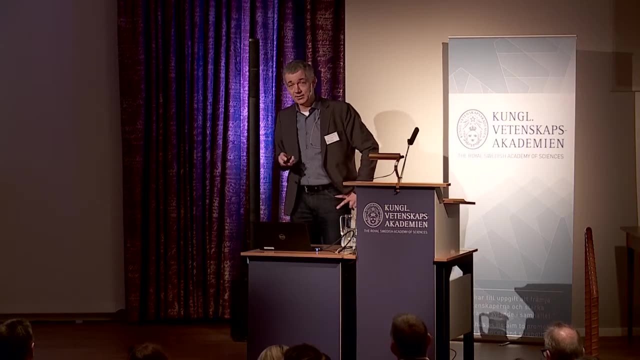 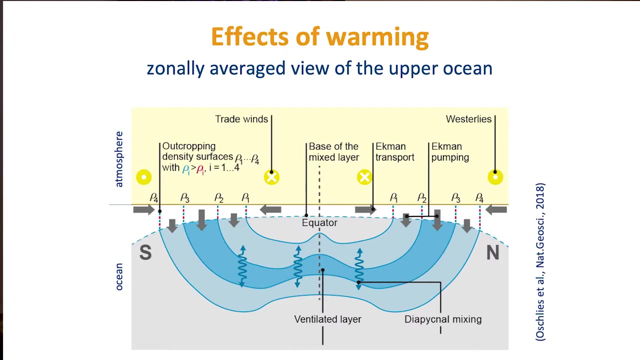 the more stratified thermocline in the warm environment. Thank you, So that's a question mark And we can now look at that in our models, And the first conceptual picture that we derived and formed by numerical modeling is here. So this is. 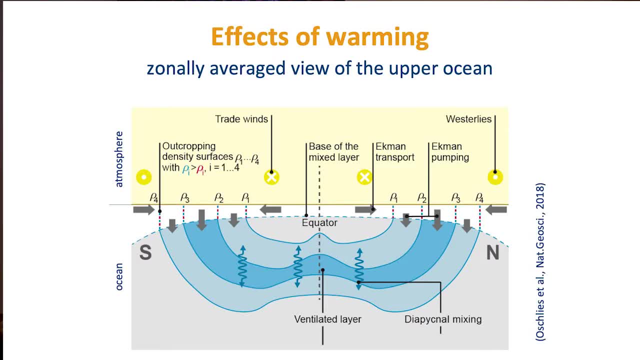 a transect through the ocean from south to north, in the middle of the equator, And the thermocline is shown, So the upper few hundred meters really, in this picture. This is the world before warming, and once we warm, Everything becomes warmer. So the red lines here And everything is more stratified. So all the 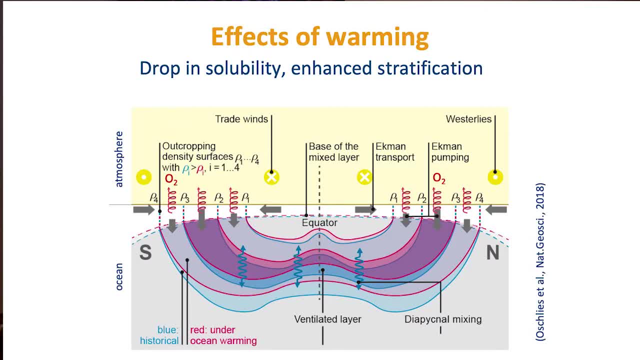 isopiginals will move up a little bit and move poleward. This is the enhanced stratification effect. There's another effect: less mixing them, Because the density stratification is sharper And we need more energy to stir it, And for the same level of energy put in by tides, by wind. 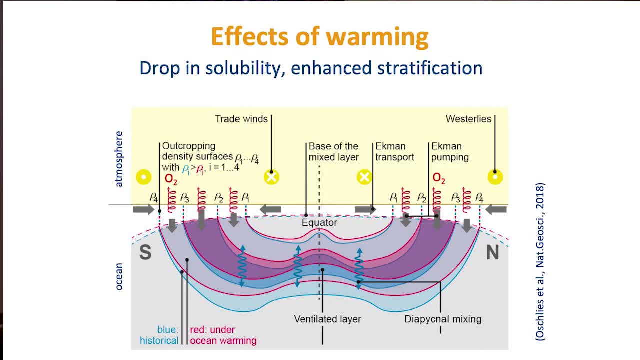 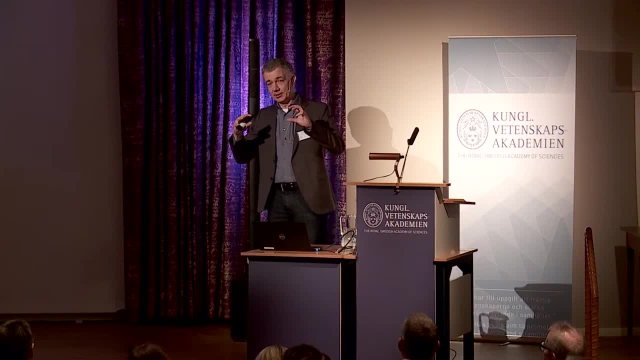 there will be less stirring, less, Less mixing. So this is an effect we see. And so all these shallow isopiginals in the thermocline move closer to the surface. They narrow down into tighter spaces, density spaces, these red ones. 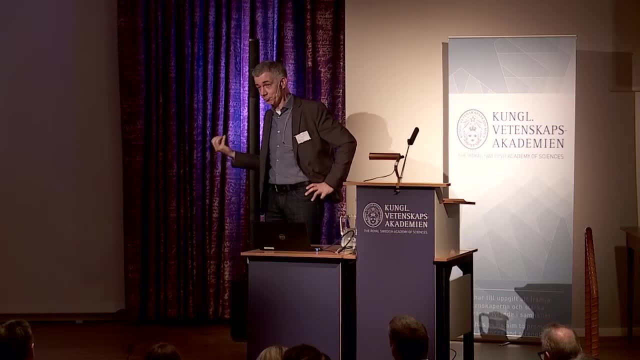 And if we have the same winds, still winds pump water with Egmont subduction, Egmont pumping And then the same transport. So the transport of water pumped into the ocean here has to move through a smaller depth horizon, So it has to move faster, So the transport velocity increases because the space that can be occupied 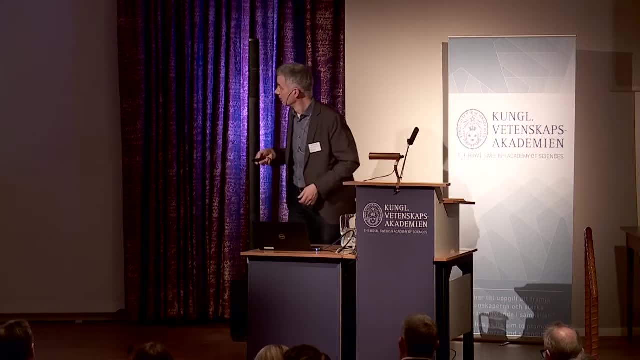 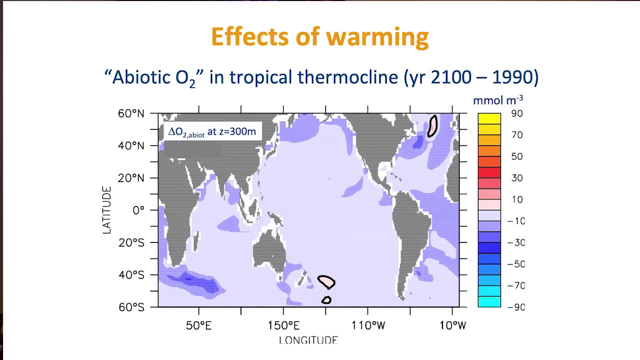 by this transport is smaller and in a warmer ocean, And so we should even see high oxygen levels, And that was one of the questions I think you referred to, And that's what we see in our models. So, first effect, this solubility effect, 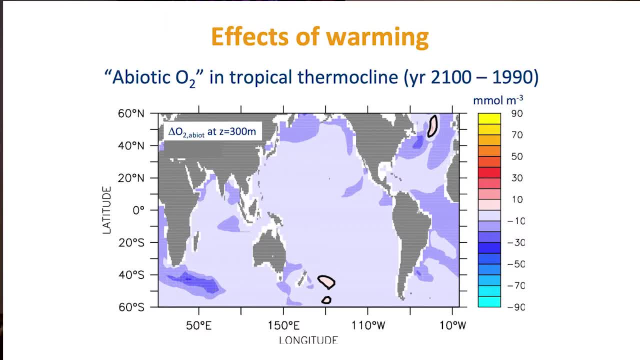 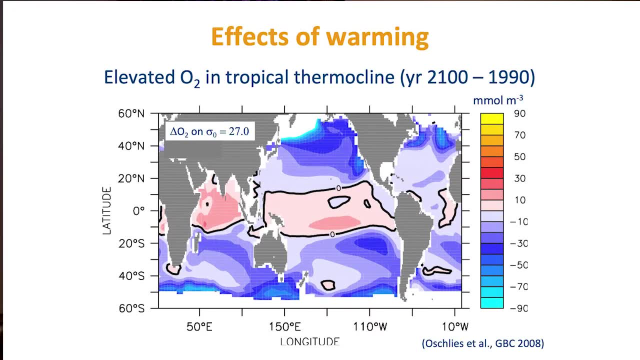 Just the gas solubility And here we can model argon or abiotic oxygen in the models And we see it goes down blue color everywhere. So oxygen levels decrease in the global ocean. But if we look into this warming effect on circulation, on transport, then the models show indeed this is for fixed winds. 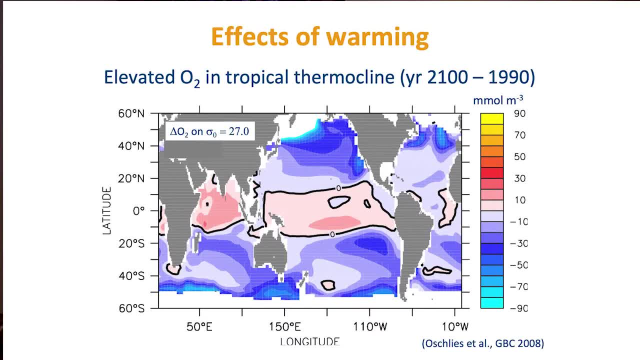 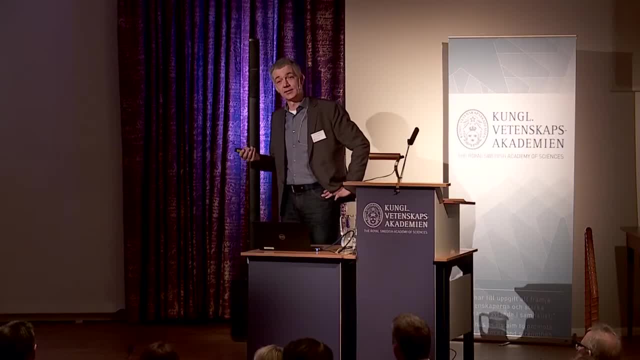 So the winds have, atmosphere circulation is kept fixed at present day values And we model just the warming effect, The enhanced stratification effect And this speeding up of subduction in the thermocline of the transport in this narrower space for ventilation, for thermocline circulation. 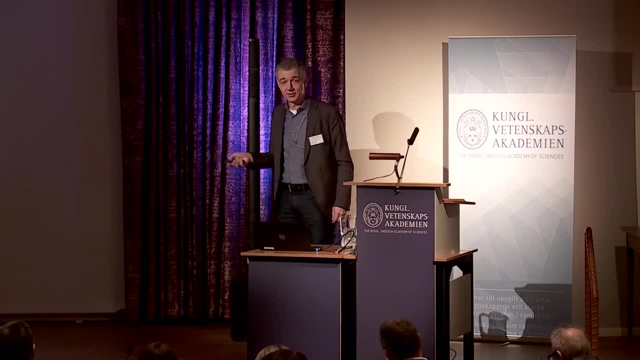 And this results in enhanced oxygen values in the tropical oceans, Because there the water didn't have enough time to accumulate the same respiration signal And it arrives with high oxygen levels Even though it has warmer, And this This exceeds the solubility effect here that we see in this warming world. 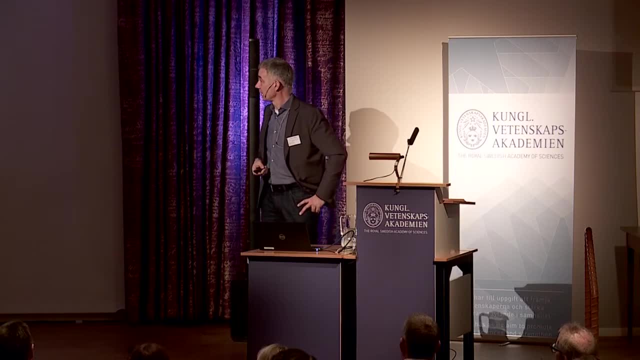 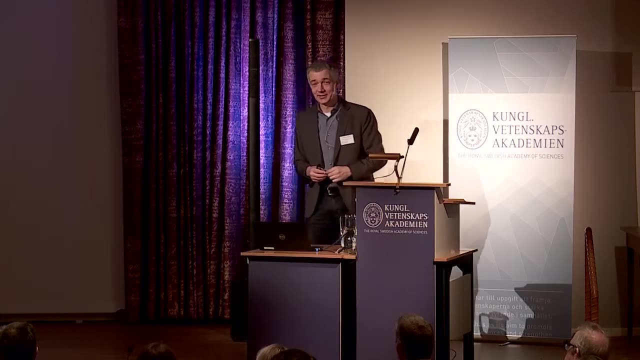 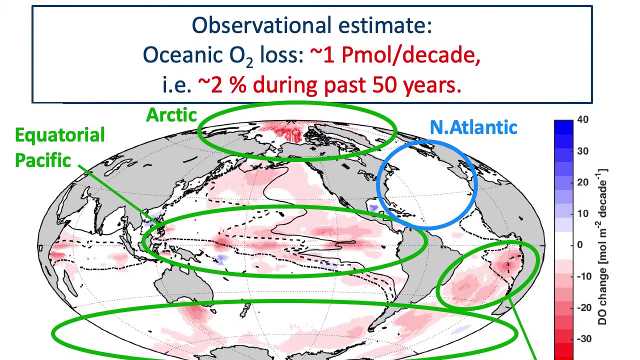 That's models, And now we have reality. And there we see. unfortunately, the color scale is now opposite. The red color here is deoxygenation, So the alarming signal that we wanted to transport, or the authors here wanted to transport. So this picture shows the decline of oxygen almost everywhere. 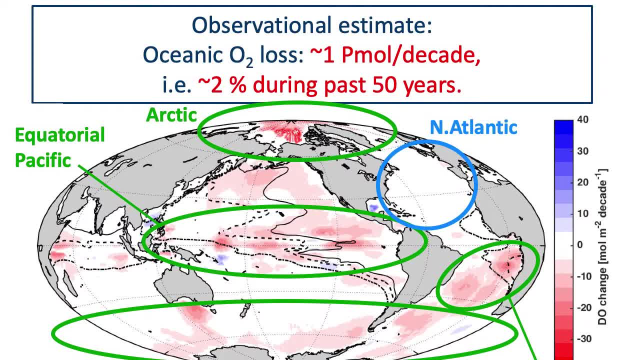 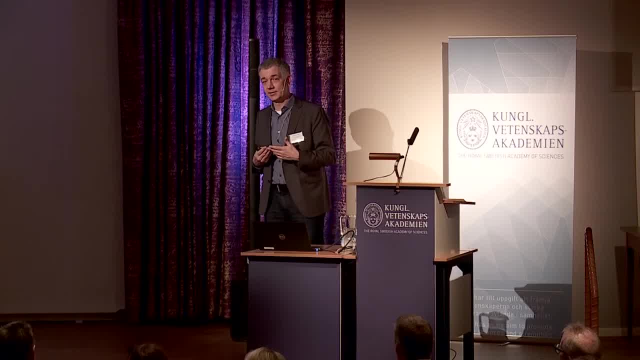 Including the tropical oceans, And that means another major change And that means another mechanism, Not only solubility and this transport effect, But also either wind effects- So changes in atmospheric circulation- Or biological effects come into play here, And this is more difficult to disentangle. 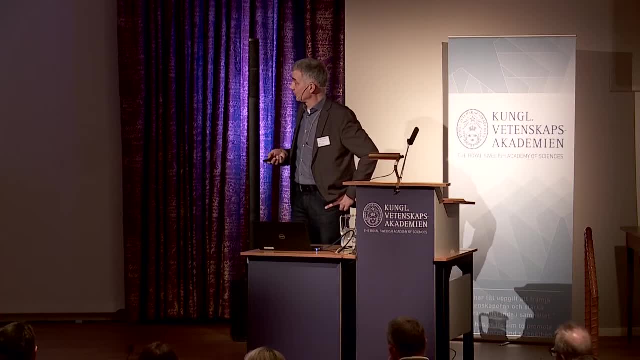 But the picture here is decline essentially everywhere And it's quite drastic. So it's 2% decline of the ocean oxygen inventory over the last 50 years. So extrapolating this into the future Would bring the ocean life to an end in 2,500 years. 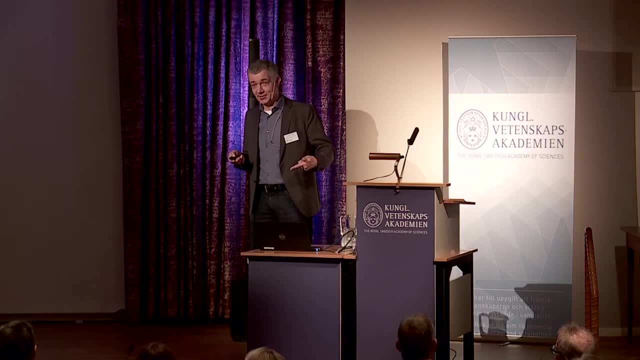 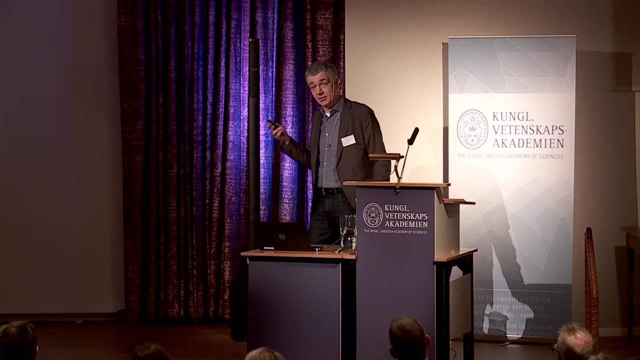 Which wouldn't be too good. But there are feedbacks from the system And I will come to a few of these. We see particularly high oxygen loss in the Arctic, So there's lots of changes going on in the Arctic, More production. 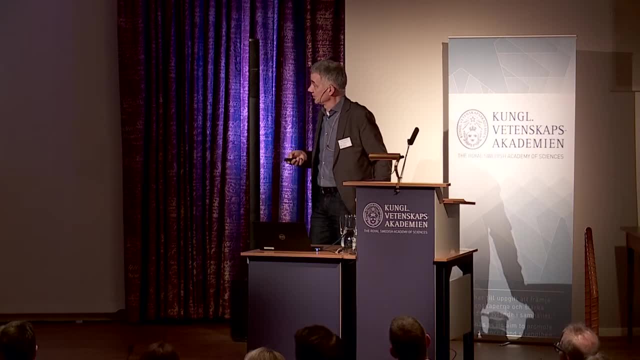 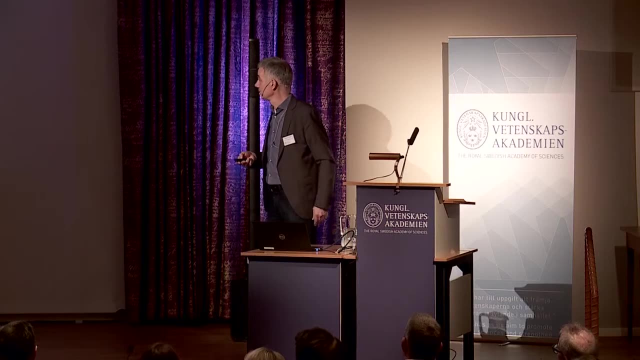 More respiration. This could be an effect here in the equatorial Pacific Southern ocean as well. Very interesting Changes going on there In terms of also carbon uptake- CO2 uptake- A very important domain- But also oxygen. This was surprising. And also South Atlantic- A surprise as well- And the data compilation. This shows up as a point of above average oxygen loss. Interestingly, the North Atlantic- Perhaps the most The best studied region in the global ocean- Doesn't show a very significant oxygen decline. 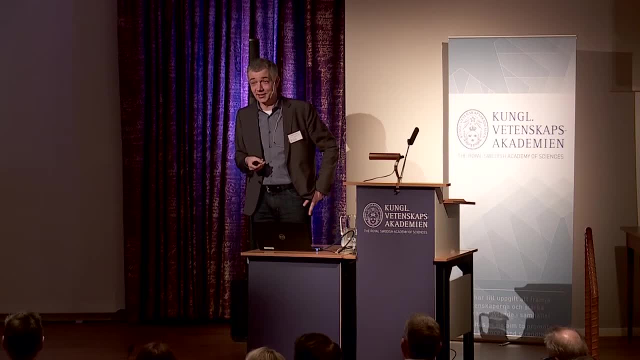 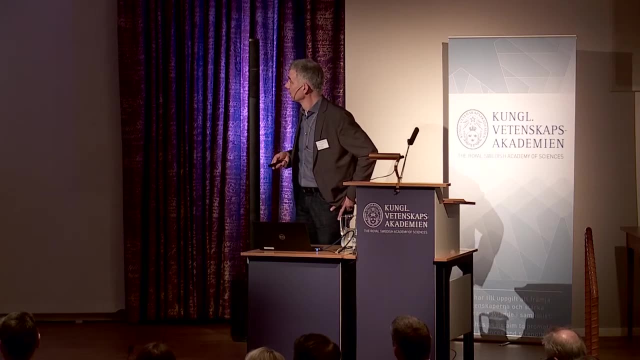 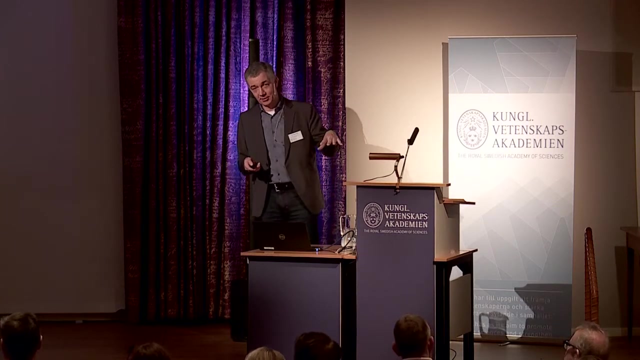 So it's, below average, An anomalous ocean basin, And so we should maybe not infer global ocean properties From studying the North Atlantic alone. So what do the models say? Now? we have seen a few model studies about processes And the global picture from data. 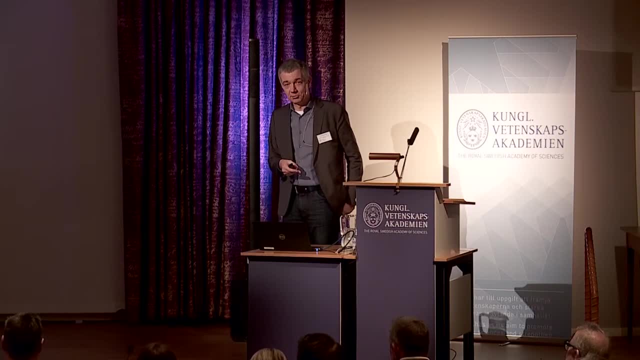 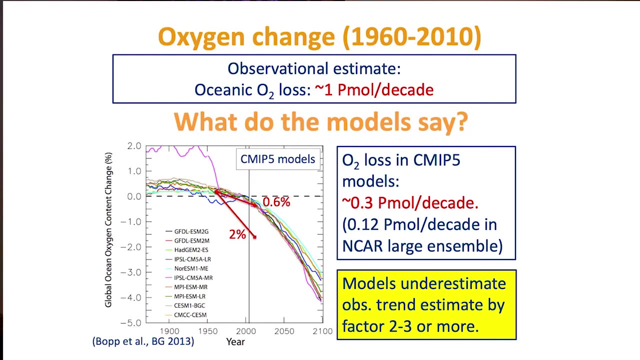 And unfortunately, the models do not at all disagree, Do not at all agree, So there's a huge discrepancy. These are the IPCC models, The most recent IPCC report, CMAP5 models, And they show all a decline in oxygen. This is up to today. 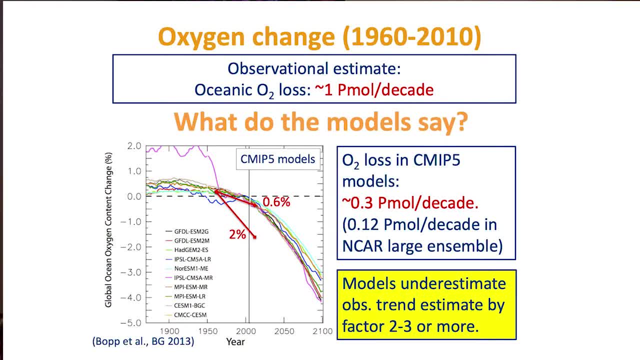 But then also for the future of the century. With increasing warming We see an increasing decline of oxygen. But none of these models gets a 2% decline, So they have a 0.3 percent decline. So that's 0.3 per decade. 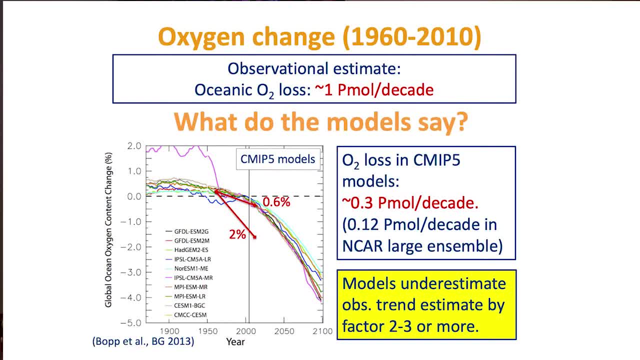 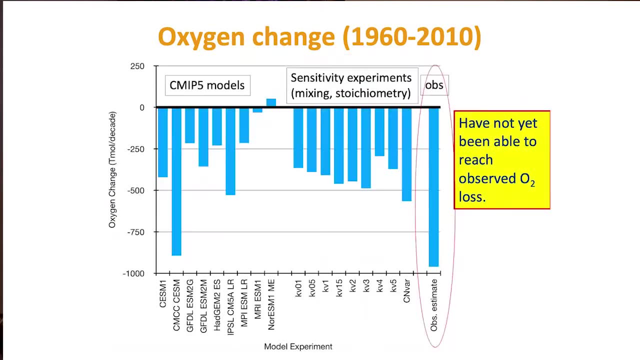 So that's 0.6%. So an underestimate by factor 2 to 3.. By essentially all the models, And this is a systematic deficiency, apparently, And we still haven't found a solution for this. So we tried. This is the observational estimate. 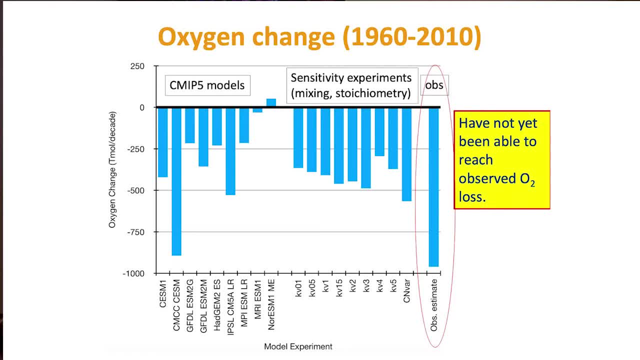 Decline over the last decades, Five decades. These are all the IPCC models. One gets close, But for the wrong reasons. This model that shows a decline in the 60s here Because the spin-up was not done long enough, I think. 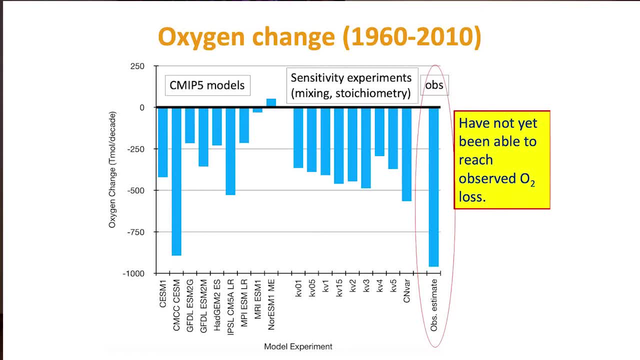 So this is an outlier, we shouldn't consider too much. But we tried also in Kiel with our models To do sensitivity studies: Changing mixing parameterization, Changing biology, Stoichiometry, Response to carbon fertilization, Many, many different ideas we came up. 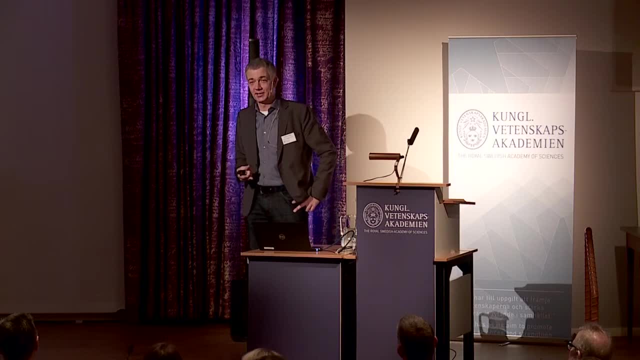 But none of them Went all the way to this 2% decline over the last 50 years. So we are still a factor 2 away, And this is a little bit worrying, Since we tried to model carbon uptake by the oceans as well. 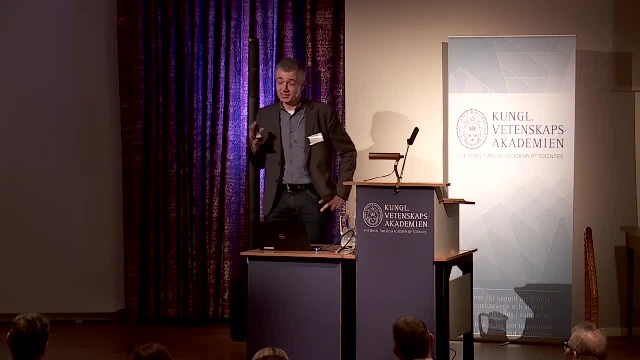 Another gas And if we are wrong there Or heat uptake. Many things We tried to model. And with the oceans We know the ocean is a key player in the climate system And oxygen is maybe an ideal tracer. We have lots of observations over the last decades. 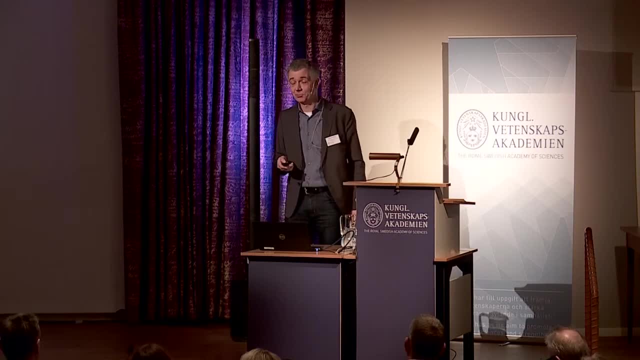 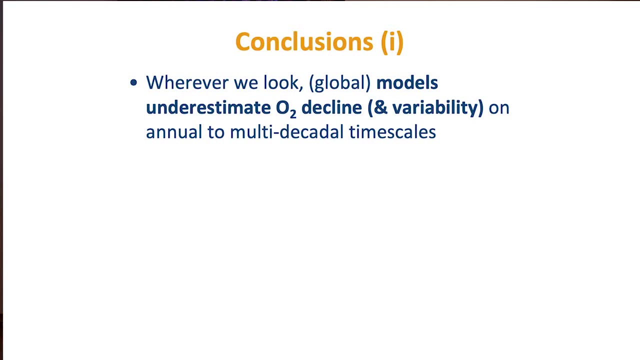 And this can be used, And should be used, To calibrate our climate models Better. So there's homework for the modelers. And well, wherever we look, Models underestimate the decline And they actually also underestimate variability, Seasonal variability. 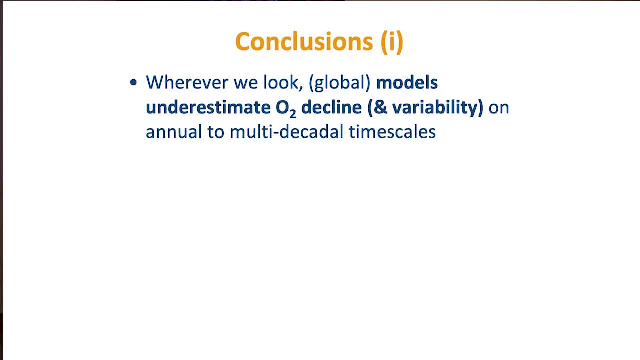 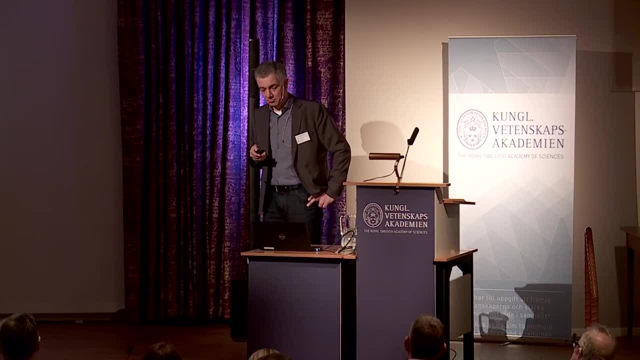 Interannual variability, El Nino variability, All the effects on oxygen are underestimated By all the best climate models, by a factor 2 or more. So this is a reason for concern, But also well, it's good that we have all the oxygen data now. 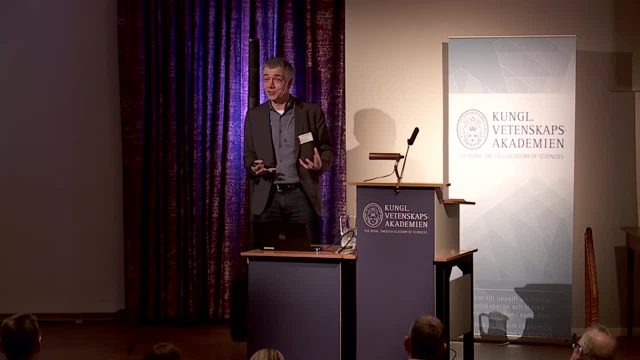 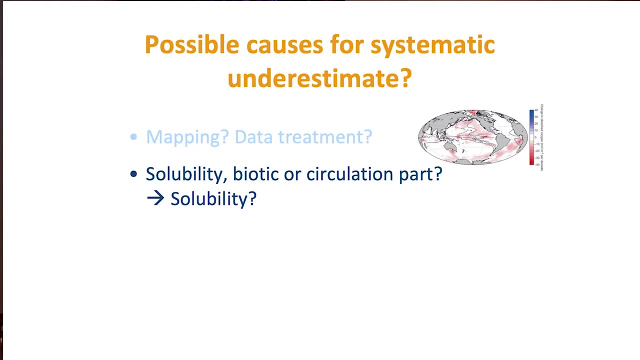 And there's more emphasis on studying oxygen in the ocean. I think it will help climate models to improve And so possible causes. Well, there are some issues about data treatment. It's still interpolating from very isolated data sources Of different quality. maybe. 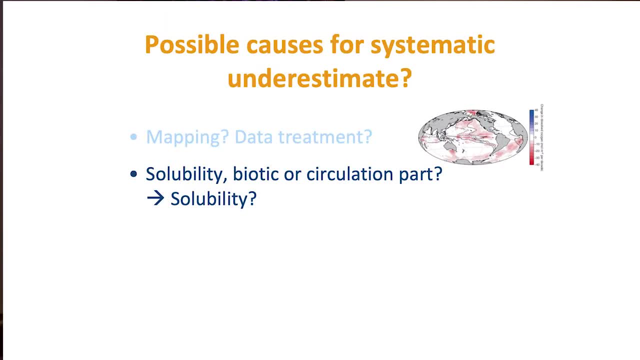 So we have to check that as well, And we are doing this. But so far we have no evidence that this is a major reason for this discrepancy Between observation estimates And model estimates. So solubility could be one reason That would be the heat uptake. 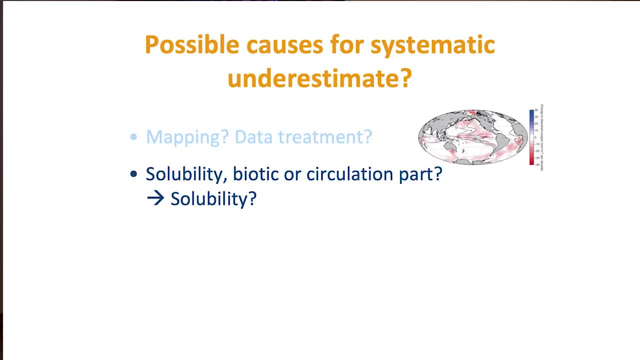 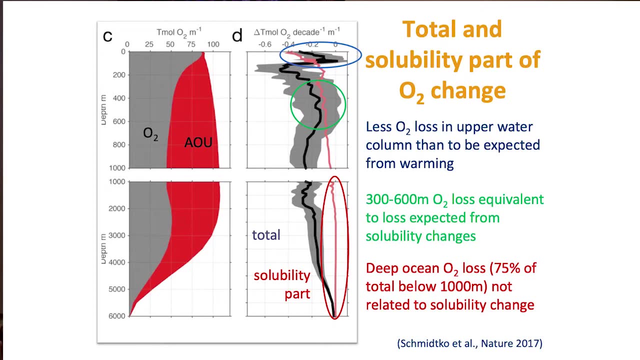 That would be really critical for climate models. Or it could be biotic or circulation parts. Looking at solubility first, From the data we see, Let's look at this panel here. This is the total oxygen decline in gray Over the water column. 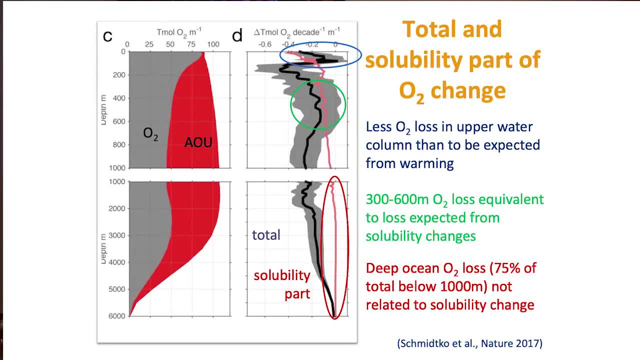 From the surface to 6,000 meters. So global ocean average decline And the red curve That's the solubility driven. So that's the warming effect over the last 50 years And we see that on the surface, The decline. 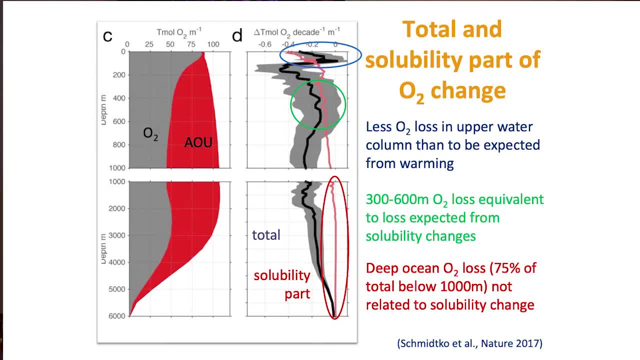 Total decline is smaller than we would expect from the warming, The solubility effect, The champagne effect. So there's some feedback. apparently, stabilizing oxygen in the surface waters Could be a reduction of respiration, Reduction of biological production, Enhanced stratification. 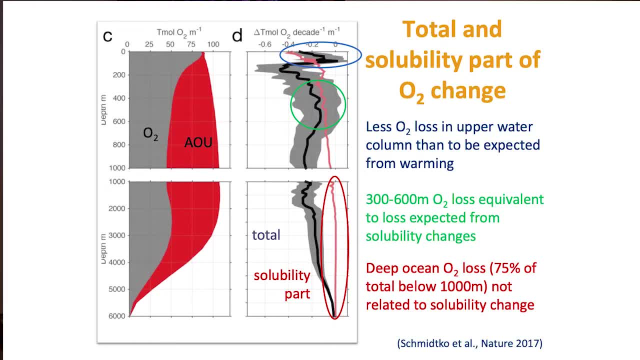 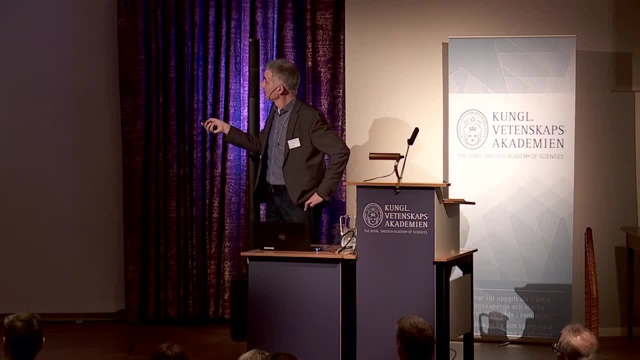 But could also be this ventilation effect on the tropical oceans, That waters move faster Through the thermocline, Then in the deeper thermocline. Essentially all of the loss is explained, Or can be explained by solubility changes, Gas solubility change. 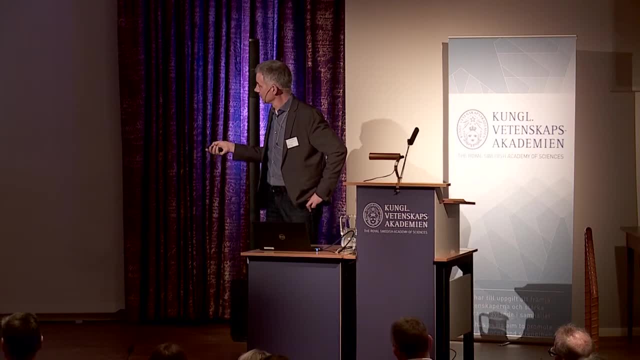 Temperature effect At depth. Almost none is explained by the red curve. So this is must All the oxygen decline we observe At deeper levels, Deeper than about 1,000 meters. 1,200 meters Is due to circulation. 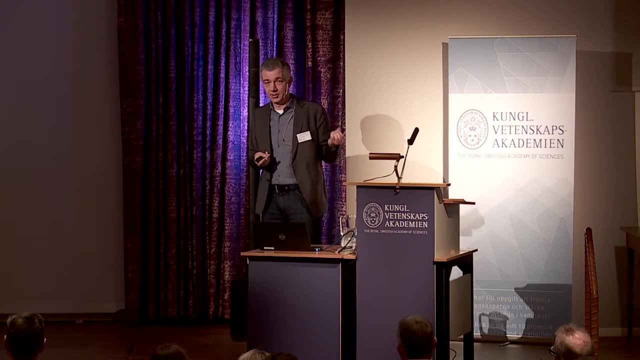 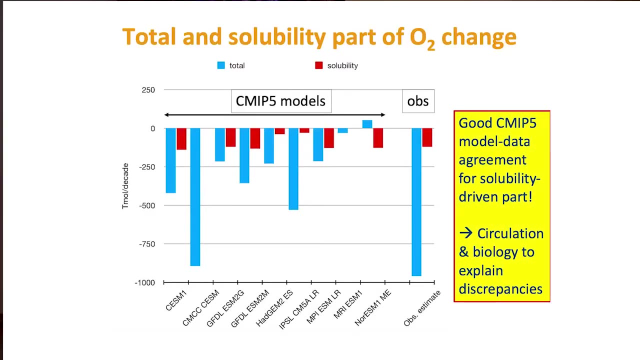 Circulation changes Or biotic effects. We don't have any other explanation for that. What do the models again say? So here are our C-MIP, IPCC models And the observational decline in blue. That's what we saw earlier. And now the red part. 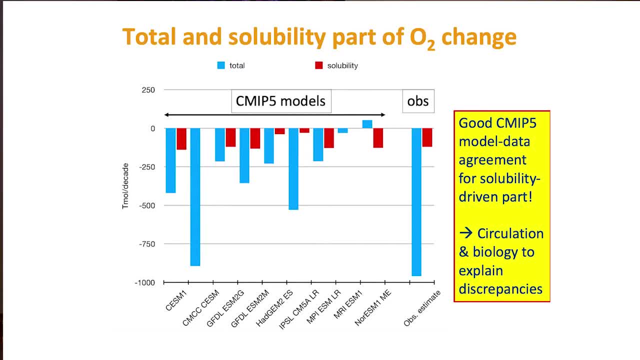 That's the solubility part Which we can diagnose from the data From the previous slide And from the models as well. And here, Fortunately, a relief for the models. The models tend to agree, Most models at least, So on average there's a good agreement. 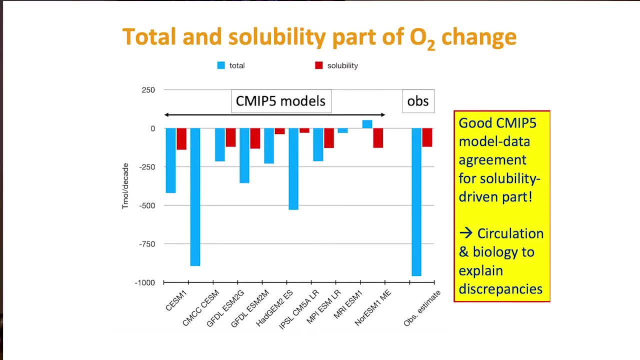 And we have models that do agree. Let's put it that way. So the red bars here are similar magnitude, Not a factor too different. And so the heat uptake? apparently There's no reason to expect the heat uptake in the models is wrong. 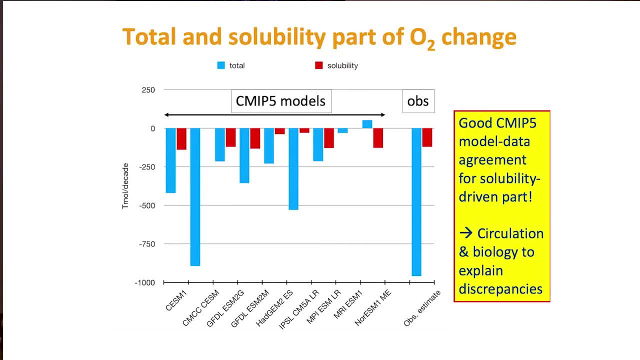 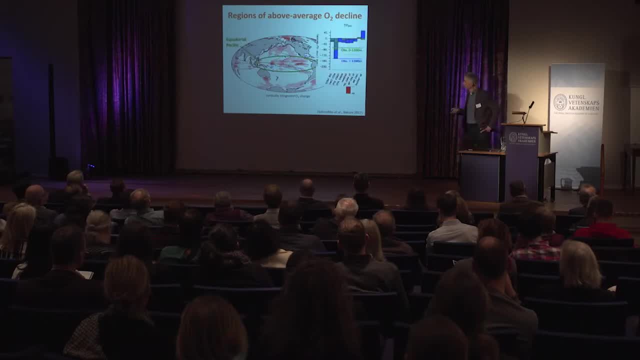 So that's a relief, I think. So it must be something else- Circulation or biology, Which is wrong, And this is the first hint. And now we can look at different regions. We did that for the equatorial Pacific And here on this. 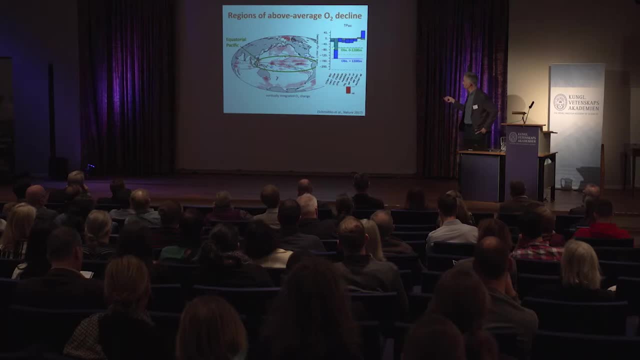 I looked at observational estimates for the upper ocean in green And for the deep ocean Deeper than 1,200 meters, The blue And the bars. here are the models. And so in the tropical Pacific, Both models are wrong, for the shallow and for the deep part. 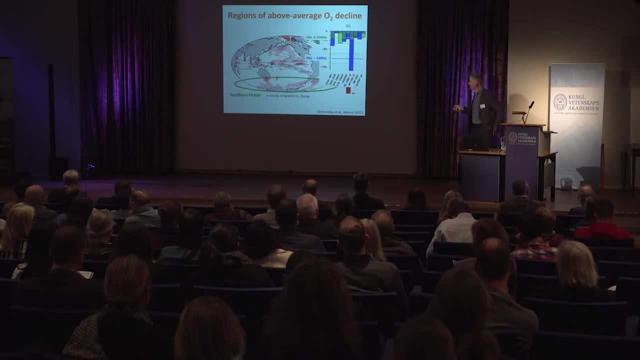 Very bad, Very poor performance. Other regions, southern ocean models are pretty good for the upper ocean, Upper 1,000 meters, But they completely miss the large deoxygenation at depth. Almost all models at least miss it. Atlantic, South Atlantic as well. 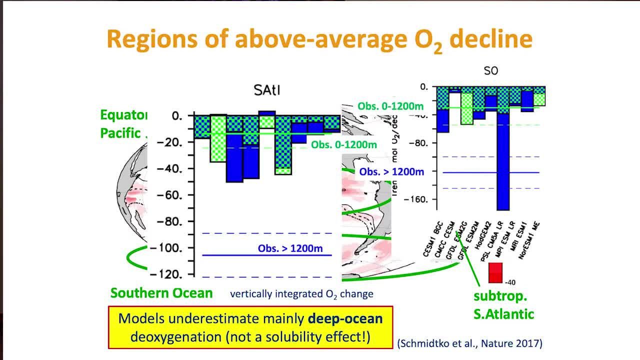 Pretty good. The green bars and green line: here They seem to agree pretty well. Out of magnitude is right, But the deep observed deoxygenation is completely missed by the models. So it's something going on in the deep that the models don't get. 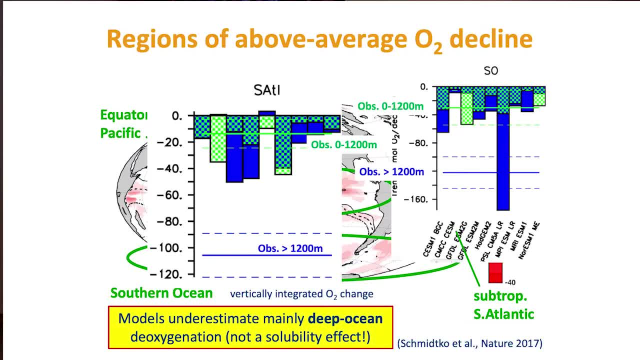 And I think this is circulation Respiration. There's little evidence for enhanced respiration at depth, Since metabolic effects will speed up respiration in the warming ocean. That means if we don't change the sinking velocity or sinking profile, Respiration will occur shallow up in the ocean. 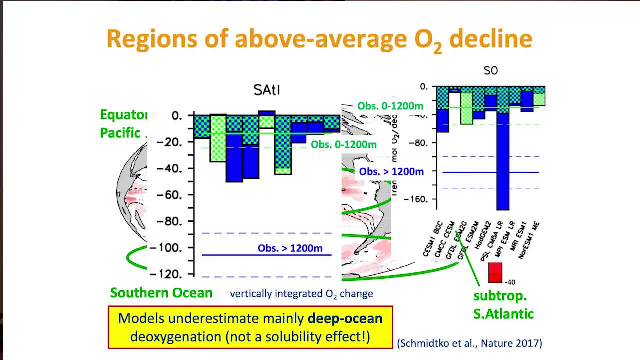 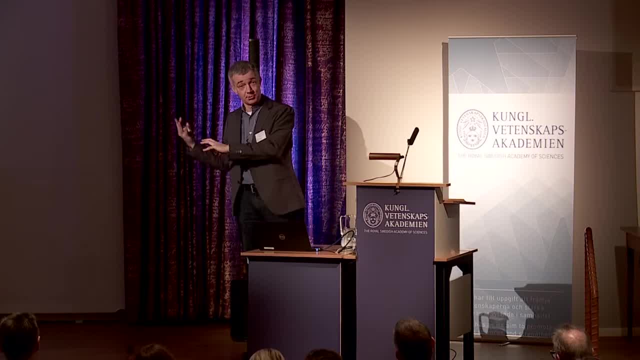 So it will enhance respiration, oxygen consumption at shallow levels, And less material organic matter arrives in the deeper ocean, And so less oxygen consumption by biology. That's what we at least see in the models Where we assume that there's no major change in the quality of particles. 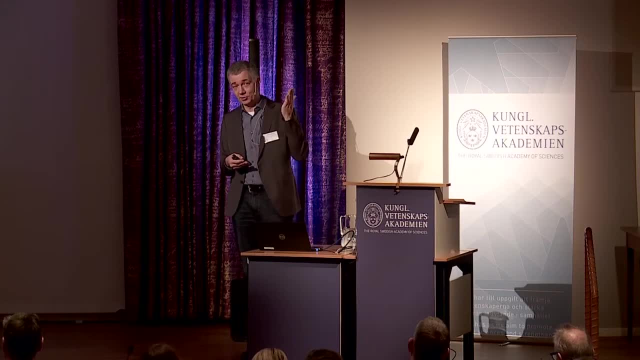 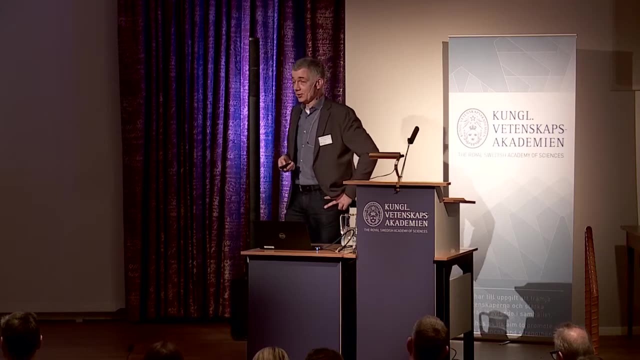 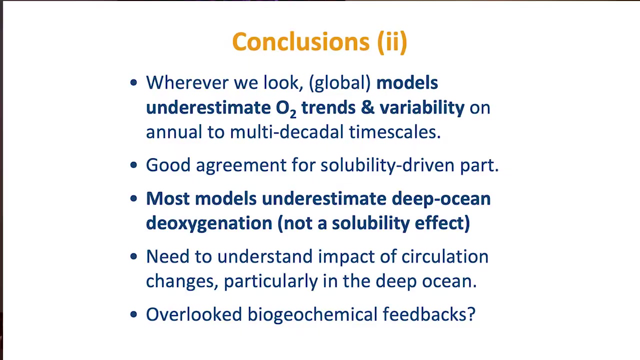 And the sinking speeds And the vertical distribution mostly of mechanical sinking. So this is apparently the deep deoxygenation. I think it's certainly not a solubility effect- That's what we have seen- But it's likely a circulation effect. 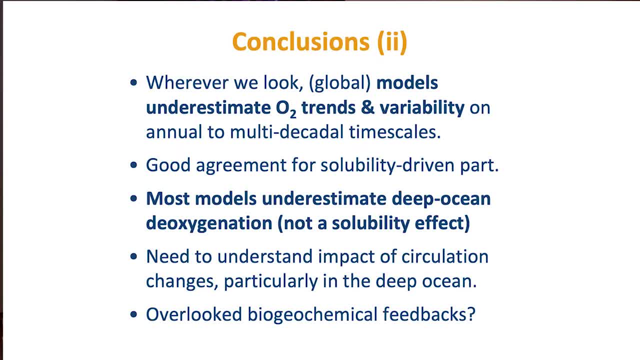 And I think this is our major conclusion we have right now That models do not get the circulation changes in the deep ocean right, If our oxygen observations of the last 50 years are right. So this is what we need: to understand: The impact of circulation changes. 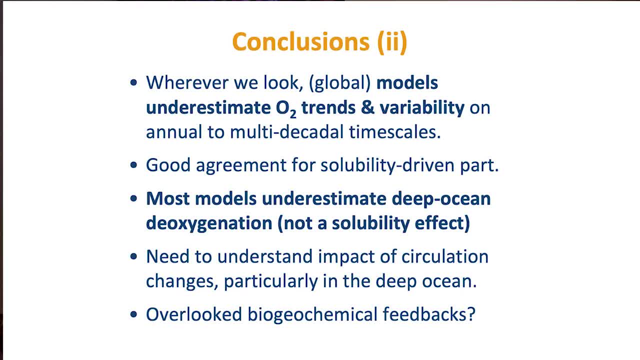 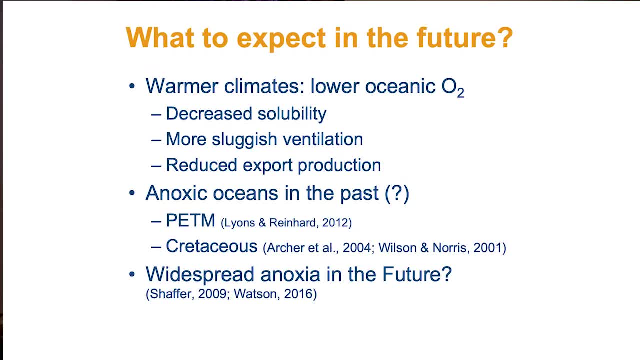 Particularly in the deep ocean. Of course, there may be overlooked biochemical feedbacks, And one of these is now came, Well, basically fall onto our feet When we tried to extrapolate, To speculate What will happen now in the future. So what should we expect? 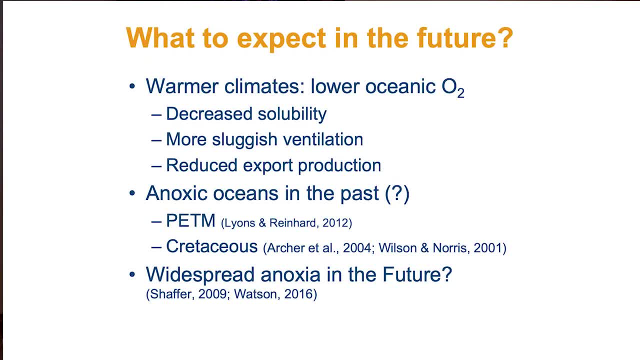 Oxygen is going down 2% over 50 years And if we extrapolate that, We also assume it gets worse with increasing warming, And right now rates of warming still increase. So we have the notion warmer climates have a lower oxygen content of the ocean. 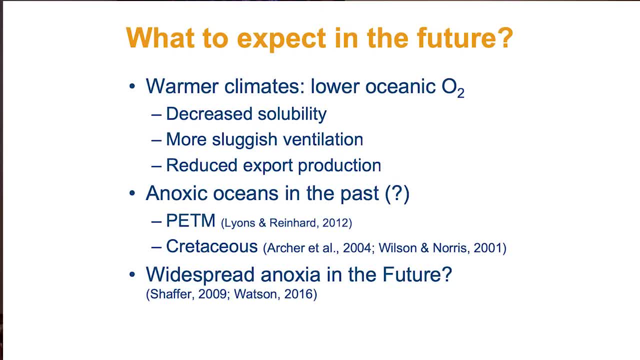 Decreased solubility. That's what we have seen on average, Probably a more sluggish ventilation for the deep ocean And maybe reduced export production. We have seen, Or we have evidence from geological records, That there were anoxic oceans, At least anoxic ocean basins, in the past. 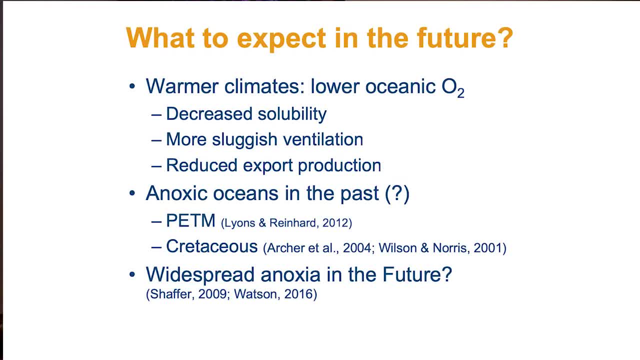 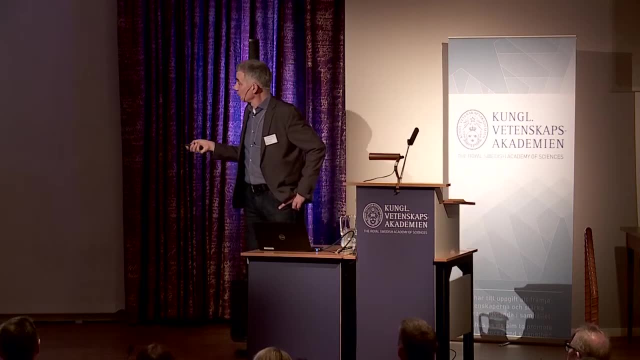 Cretaceous, PETM. And so the question is: Is there widespread anoxia to be expected in the future For the global ocean, Or for ocean basins, Maybe for the Baltic Sea? And we ran our models, Global models. 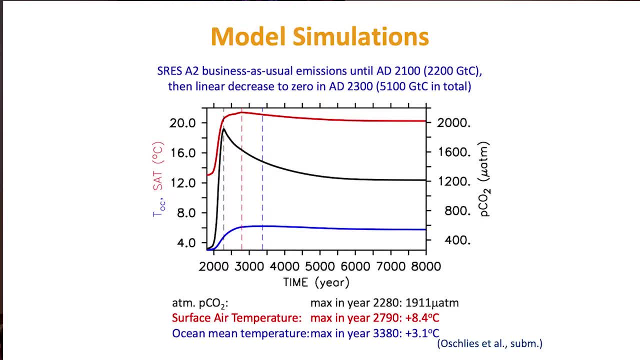 Until the year 8000.. So, extrapolating, Everything should be dead by the year 4500.. So we really did a long assimilation here And we see It's a business as usual scenario. So about 5000 gigatons of carbon will be burned altogether. 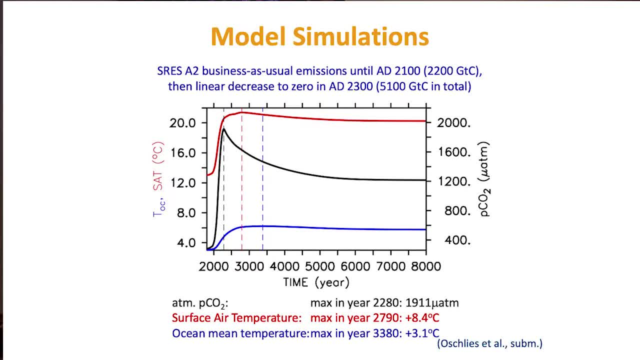 So it's still. That's the track we are on right now, If we don't change our behavior. So there's a drastic warming By about 8 degrees. PCO2 goes Peaks until everything is burned And then slowly goes down. 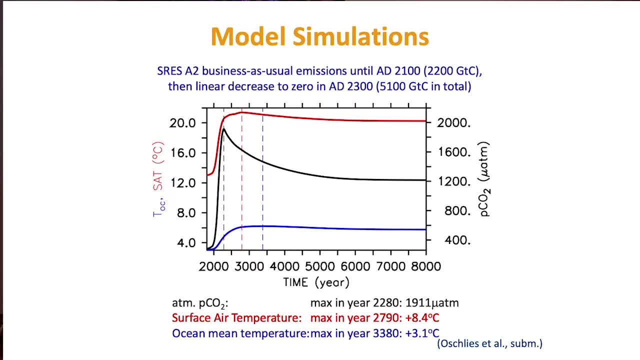 And there's no sediments in this ocean, So the real decline might be a little bit faster Once sediments- Calcium carbonate sediments- dissolve. This is not included in the simulation And the average ocean temperature goes up by about 3 degrees. 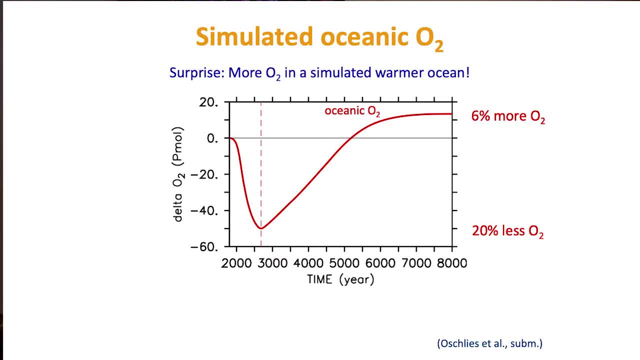 So average global ocean warming. Surprise We see oxygen levels in this warmer ocean at the end Are even higher than they are today. So we have a 3 degree warmer ocean average But 6% more oxygen in this ocean After some. 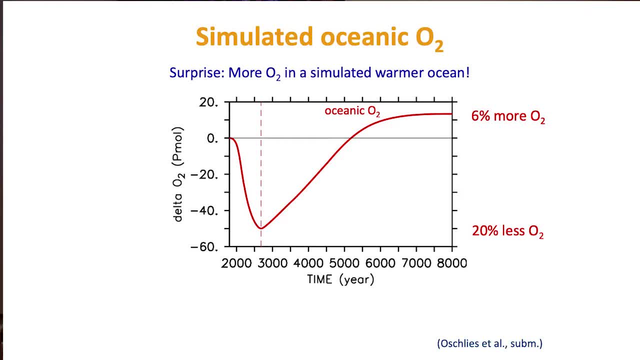 Well, crisis period here. So for the next few hundred years In our models Oxygen levels really go down And we end up. The minimum here is 20% less than today. Solubility part: We can simulate that easily. So that's the 3 degree warming effect. 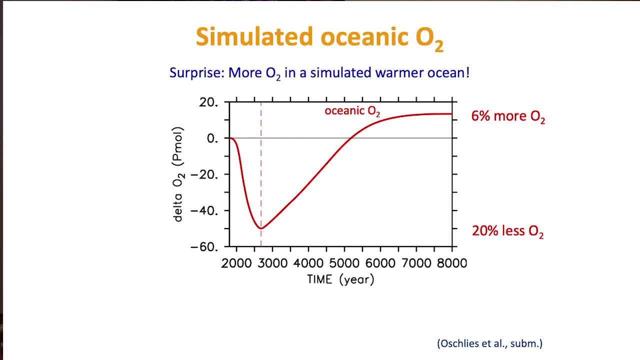 And that leads to about 10% decline of the solubility Of argon concentrations, Abiotic oxygen. But the surprise is really, In the end There's more oxygen in the ocean. So how come Is it reduced oxygen consumption? 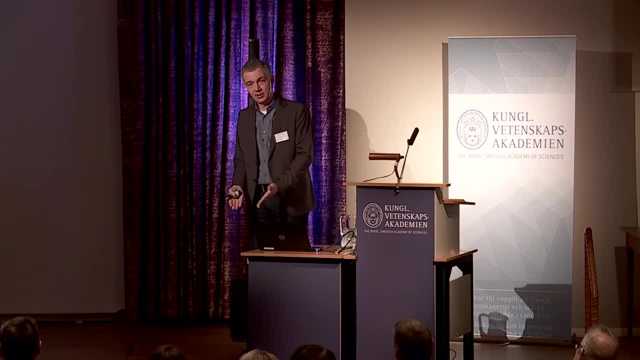 That might be an effect That we shut down biological production, So less respiration. This is not really the case. We see Well, biological production, We have here net community production, So that's basically What is available for export Or for fisheries. 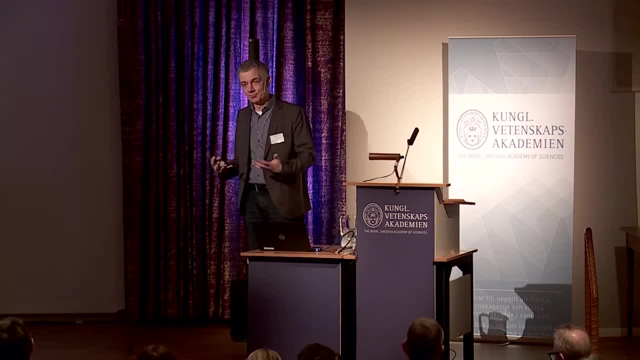 So everything, Every net surplus Of organic matter. It goes down The next few hundred years By about 10. 20%, But overall It still increases. So the Arctic Becomes more productive And circulation Rearranges. 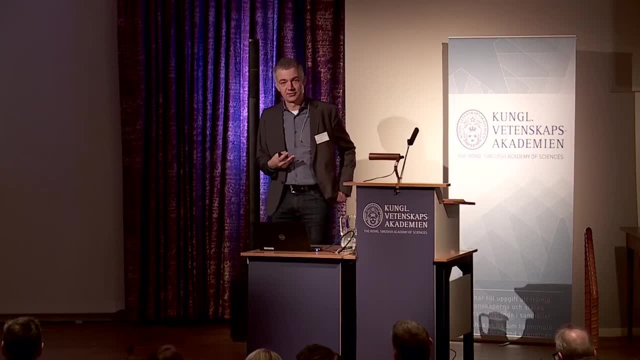 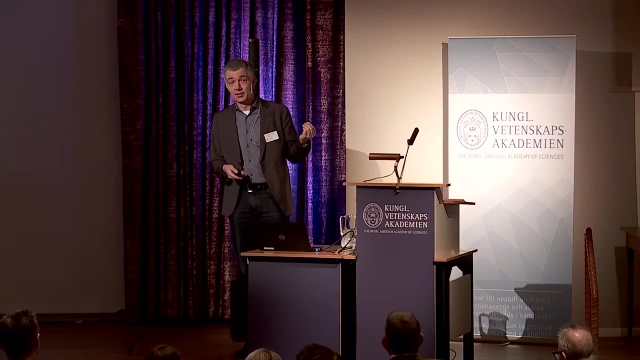 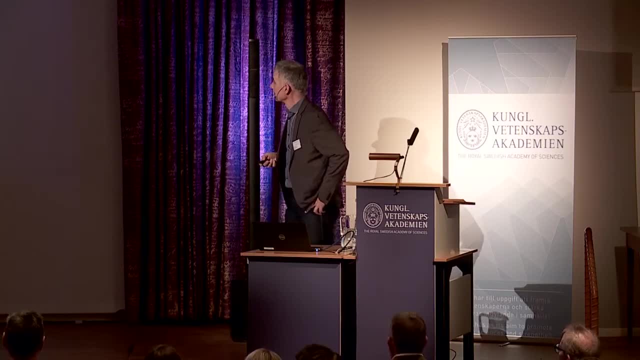 And more oxygen And more oxygen And faster Utilization Of nutrients. So This is Would even point To less Oxygen, Because More is produced, More will be Respired. How come That we have? 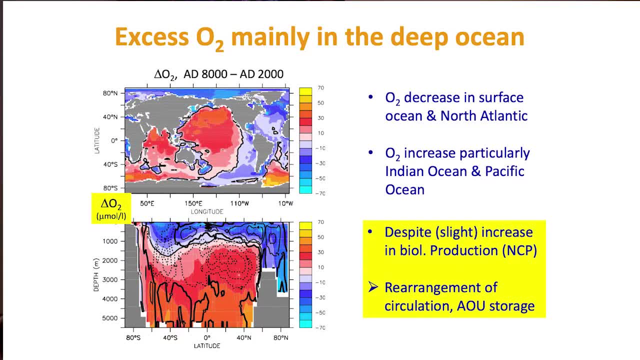 More Oxygen In this Warmer ocean And if we look At the patterns Here Again, In our model World Of Red Is always Positive One. So we see Depth Section Here. 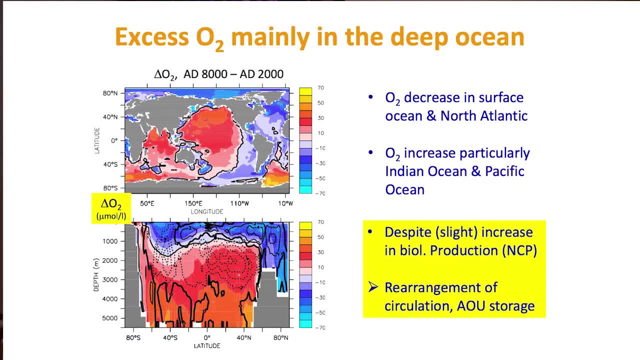 That's All Zonal Average. The ocean Shows Particularly The deep Ocean Is enriched In oxygen In this Warmer world Surface. Surface Ocean Goes Down. So that's Mostly. 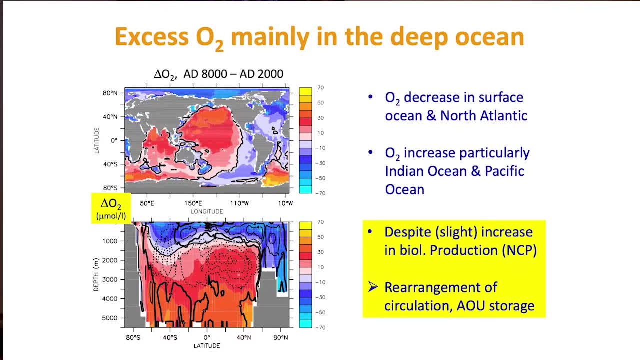 The solubility Effect, The warming Effect, The surface Waters Can Pass To Us. So, Despite This Increase In biology, Net Community Production, Despite The warming And Despite 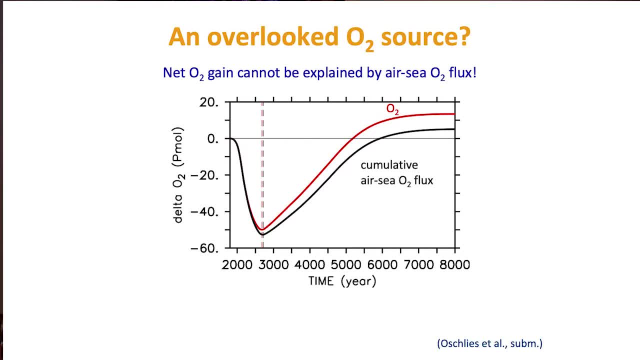 Also Some Overall Slow Down Of Circulation. We See More Oxygen In The Global Ocean And This Took Me About A Year To Figure Out. 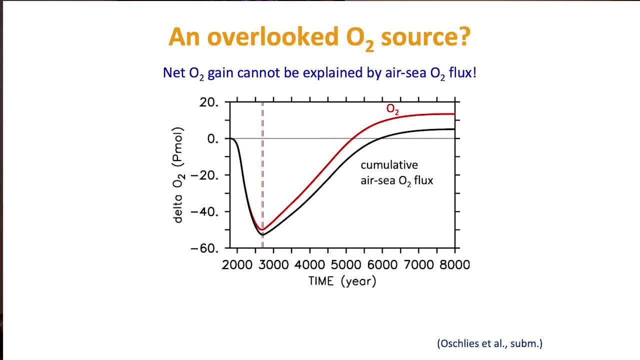 That This Was Not A Computer Bug. Well, There Were Many Computer Bugs. I Found On The Way That Atoms- And Usually We Do It- 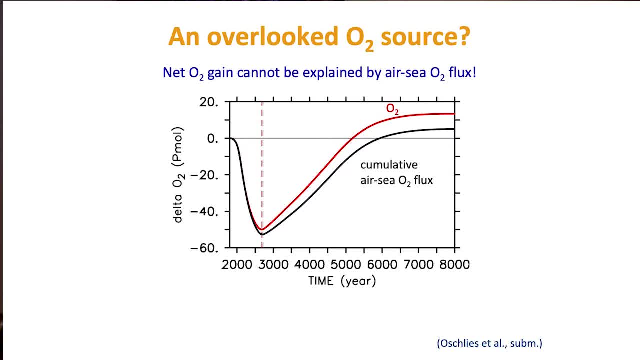 For Phosphorus. That's Our Main Currency, But But Here I Did It Lots Of Oxygen And Was Puzzled Because The Oxygen Changed The. 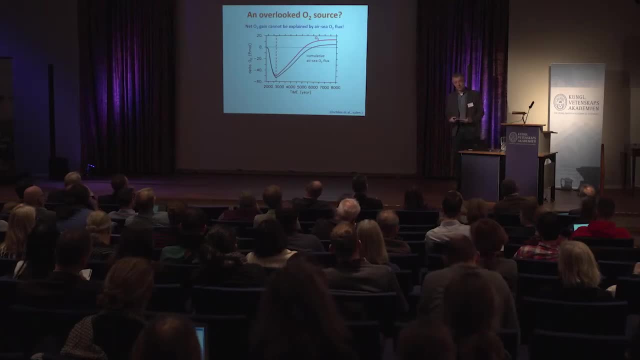 Outgassing From The Ocean, Because The Ocean Oxygen Decline, So It's We Can Breathe A Little More Oxygen. Well, Oxygen Levels In The 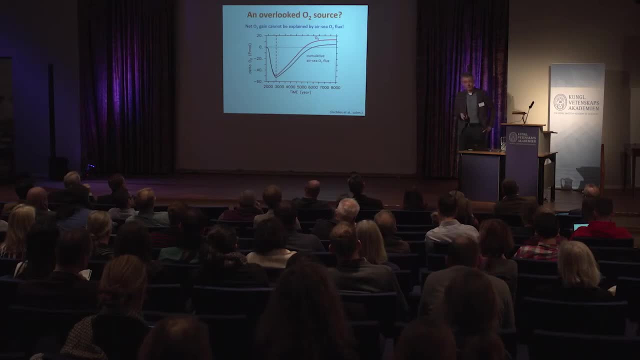 Atmosphere Still Go Down Because We Must Be Some Some Oxygen, Inferior Ocean Oxygen Source, Which I Didn't Think Of When I Drew This. 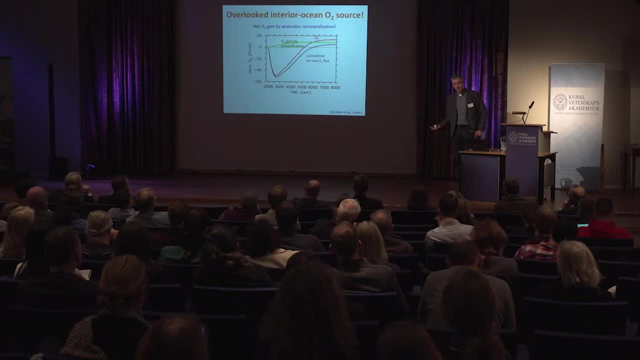 Figure And Indeed It Is The Oxygen Gain By De Notification. So De Notification Is: Is A Source Of Oxygen, A Nitrogen Fixation Synch. 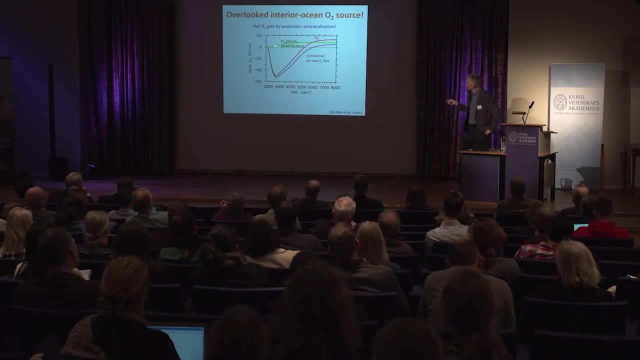 Of Oxygen, Nitrogen Fixation Plus Notification Of The Ammonium In The End. So When You Complete The Oxygen Volume So That These Regions Do, 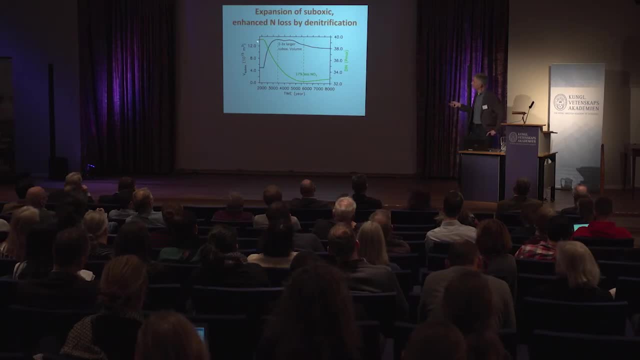 Expand Two To Three Fold In This Warming World, In Our Model World, And This Leads To Net Decline Of Nitrate, The Nutrient In 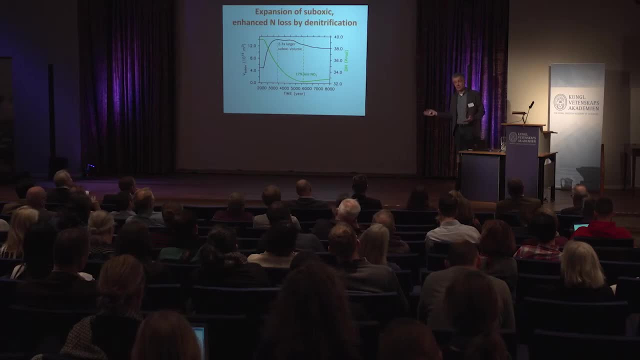 The beaucoup Of Nitrogen Most In Our World And The Nourishment Of Nitrogen And Nutrient In Our World. In The World, Nutrient In. 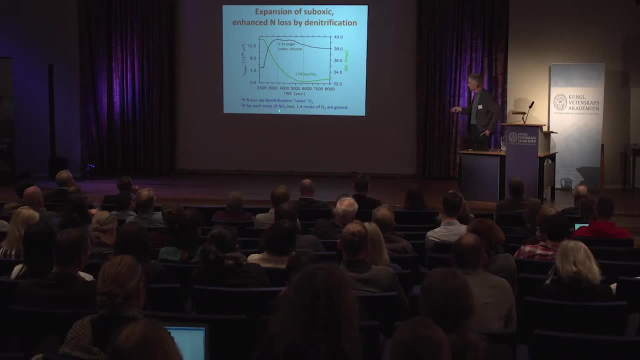 Our World Nutrient In of nitrate lost yields 1.4 moles of oxygen, because respiration does not use oxygen directly, it uses nitrate and so it's a leftover. it leaves over oxygen, it leaves behind oxygen. 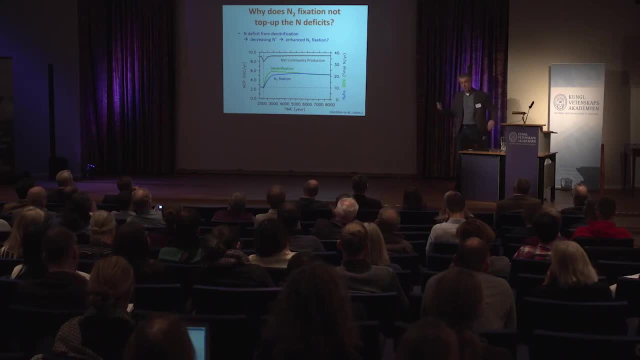 And while we have denitrification, usually we think this will enhance nitrogen fixation- in the end they are stabilising feedback in the ocean and the world, otherwise we wouldn't be here. So why does nitrogen fixation not pick up? We see the time history here. well, first, net community production evolves, goes up. a little bit. denitrification goes up quickly with expanding low oxygen environments, But nitrogen fixation has a hard time to really close this feedback to respond, and we always thought this would be a A stabilising feedback. whenever we denitrify, the ocean produces nitrate deficits still. phosphorus is around and nitrate deficits can be topped up by nitrogen fixation. That was my notion at least, that in the end, in our models, phosphorus is the key element and the nitrogen cycle is just a slave of the phosphorus and nitrogen fixers and denitrifiers. will benefit. I don't want to battle it out, but here they don't. for a few thousand years- This is about the overturning time of the ocean. so they should have enough time to really respond to see: hey, there's a nitrate deficit. maybe a better ecological niche. 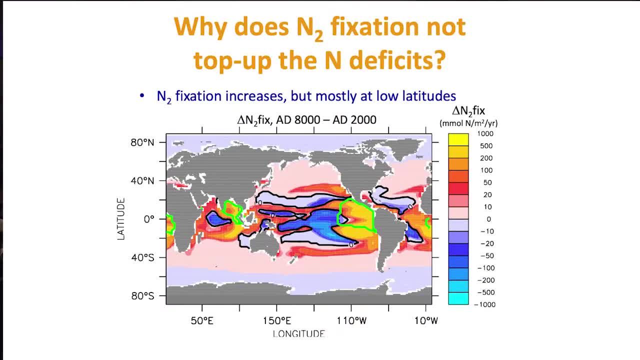 This doesn't seem to happen, And this is maybe well, the most exciting part. it's how the nitrogen cycle can have such a large, long cycle. It's a long-lasting imprint on oxygen, So we see changes in nitrogen fixation rates. 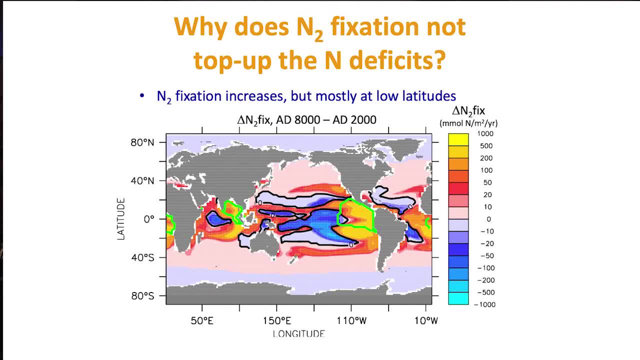 This is a global map of nitrogen fixation in year, 8,000 minus today. So we see red colours are expansion here, more nitrogen fixation. They move a little bit poleward and in both Atlantic Pacific Indian Ocean all oceans show the same figure. 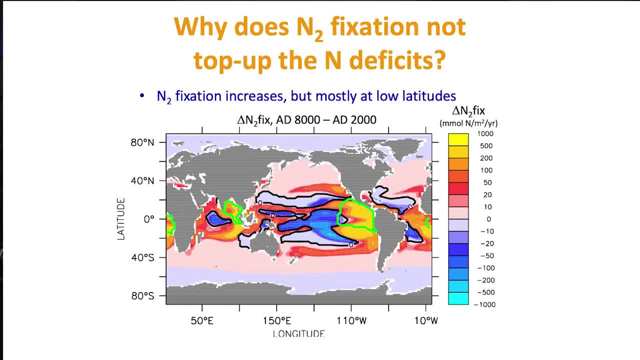 There's a little bit less nitrogen fixation Because oligotrophic regions expand, so there's also less phosphorus available, But overall nitrogen fixation increases mostly at low latitudes. That's where nitrogen fixers in our models or in our assumptions we have, we put in about. 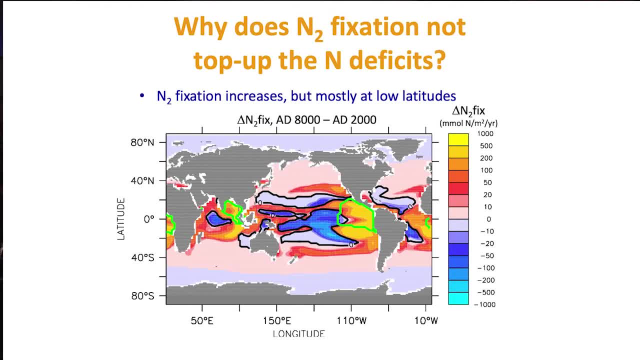 nitrogen fixers can thrive, So they have oligotrophic regions where other phytoplankton cannot compete anymore. These are usually regions low in nitrate Because again, other phytoplankton is limited then And diacetrophs- nitrogen fixers- grow more slowly. They need more energy to get rid of all the oxygen and they have more expensive machinery to run. So on average they grow about two to three times slower than an ordinary phytoplankton, And the result is that this what we call N star. 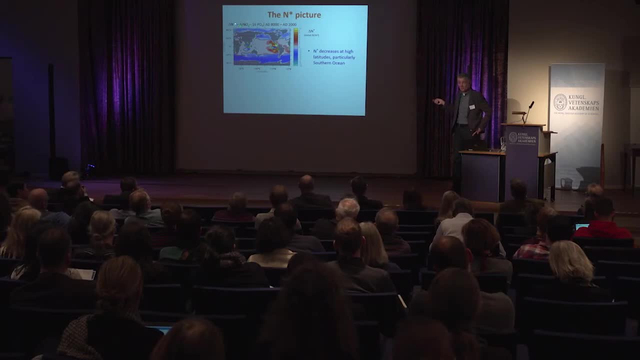 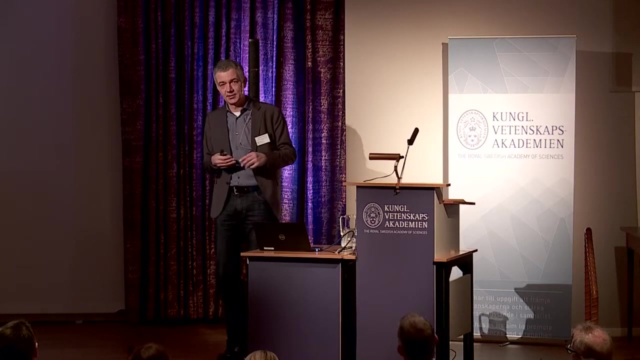 This is the difference. It's nitrate minus the red field equivalent in phosphate. so basically the excess or deficit of nitrate compared to phosphorus units. When this is positive, there's a surplus of nitrate. So it's really bad for nitrogen fixers, because then other phytoplankton can grow as well. 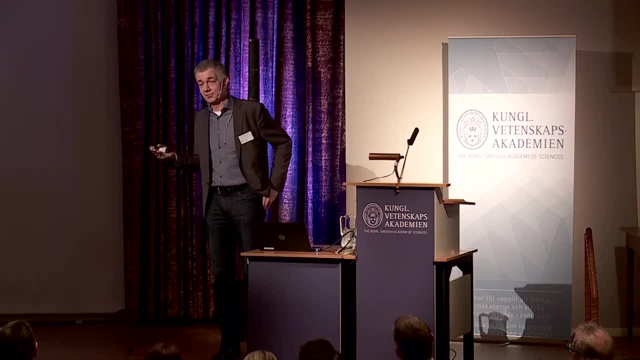 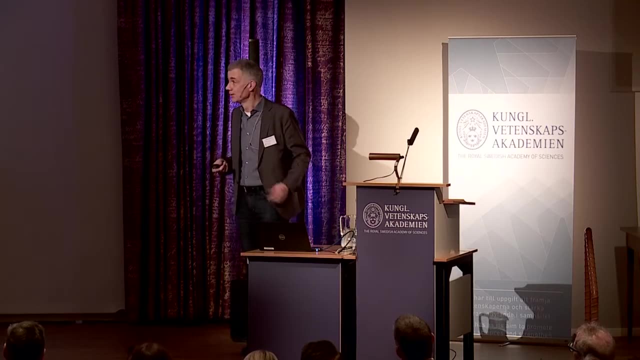 When N star is strongly negative, there's a nitrate deficit compared to phosphorus, And then the ecological niche opens for nitrogen fixers, According to our notion, Our nitrogen fixation response to environmental change. And so we see in the model the N star becomes very, very negative at high latitudes. 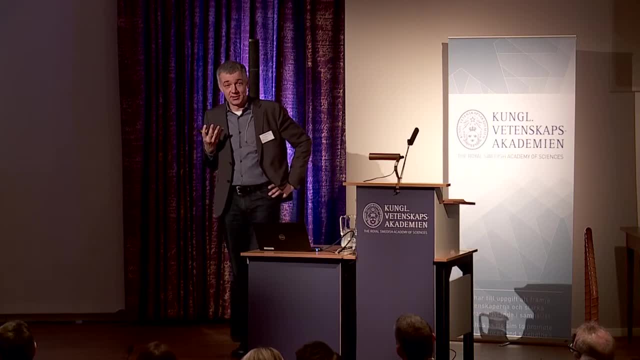 So it should be a very good environment for nitrogen fixers to top up this nitrate deficit. They top it up in the tropics, so this is about close to zero here, with some local anomalies due to upwelling of denitrification signals. 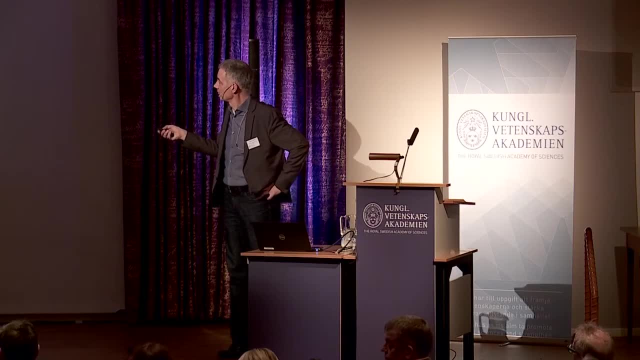 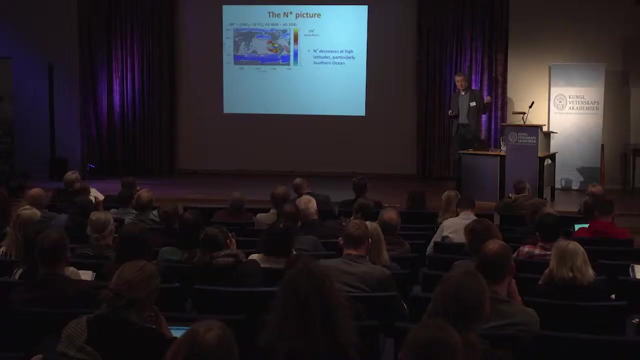 And also strong seasonal nitrogen fixation. But in high latitudes, N star, this nitrate deficits really. they grow and seem to accumulate. High latitudes are also the regions of deep water formation. even in the warmer world There's still ice, so it's still a freezing point, particularly mainly in winter. even in the Arctic there's still winter ice, So it's still freezing point, particularly mainly in winter. even in the Arctic there's still winter ice, So that's where waters become very cold. they're still salty and they sink to the deep ocean. And so these high latitude regions, they fill up the entire ocean with nitrate deficit waters And for some reason, the nitrogen fixers they can't grow, at least not fast enough in these high latitude waters to basically top up the nitrogen deficit. 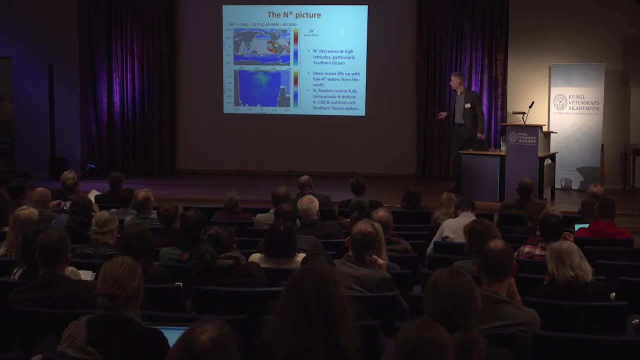 in these critical supply regions of deep ocean waters In our models. this is because we- well, that's what we told the model- Nitrogen fixers. they can't grow at low temperatures that we put in the models, so they can't grow. at temperatures colder than lower than 15 degrees. They are limited by iron that scars at high latitudes, And so they don't have a good chance really to thrive in these high latitude areas, And that's, I think, what explains why nitrogen fixers can't really respond to increased levels. of denitrification. we see They can't match. they can't grow at high latitudes where deep waters form and where this nitrate deficit can basically, via a loophole, move from the denitrification areas in the tropical regions where they will leak into the southern ocean or part of this leaks. 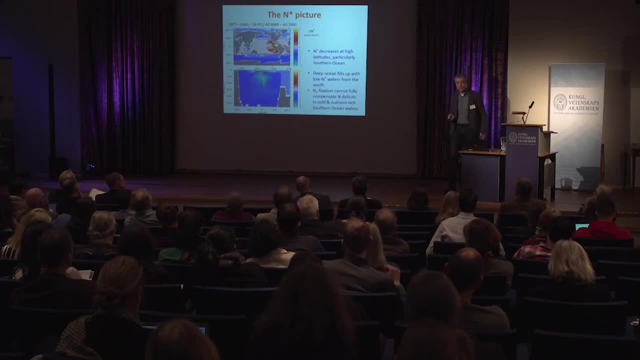 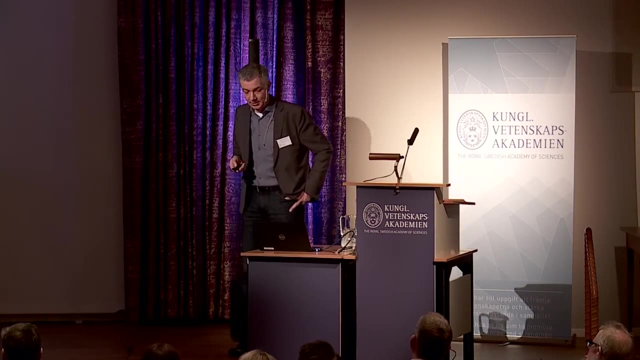 into the southern ocean and they are subducted into the deep ocean interior and fills up over long, well, millennia, fills up the ocean with nitrate deficits And so they can't, they can't really expand the oxygen deficiency and they can't reach. 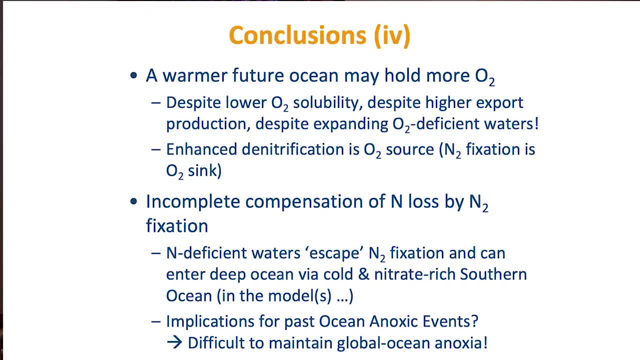 the oxygen deficiency levels. And so you know they can't. they can't be just as efficient as the surface waters. So this is the story we have about the future. A warmer future ocean may well hold more oxygen, despite lower solubility in this warming world. 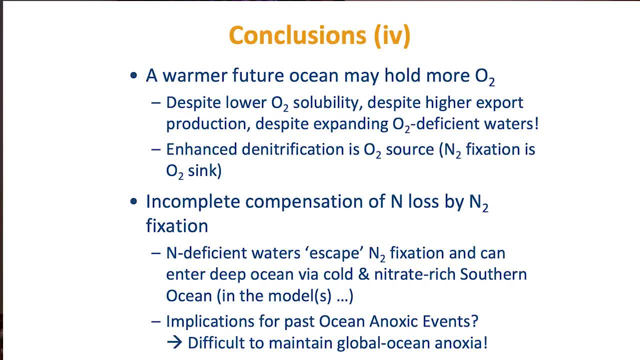 despite higher export production, despite expanding oxygen deficient waters And so enhanced denitrification, enhanced nitrate consumption in these warmer oceans is the net supply of oxygen And this seems to counter effect and even overcompensate the loss in these expanding oxygen deficient waters.